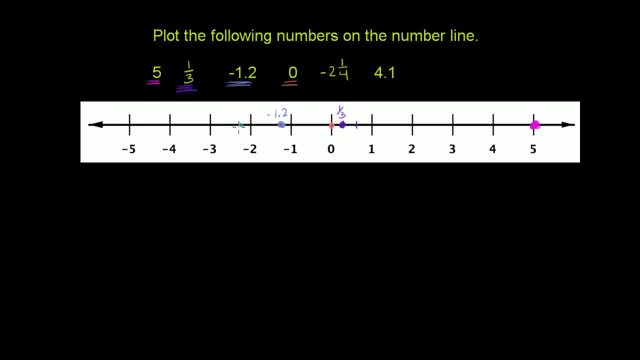 1 fourth of the way to negative 3.. So negative 2 and 1 fourth is going to be right over here. So negative 2 and 1 fourth. And then, finally, we have 4.1.. So 4 is right over here. 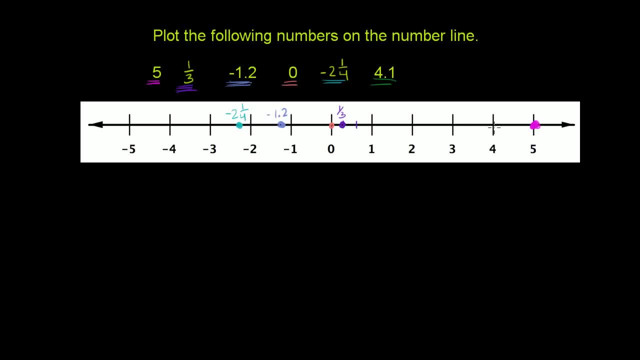 0.1 is another tenth greater than 4.. Another tenth on the way to 5.. So 4 and 1 tenth is going to be right over here: 4.1. And we are done. 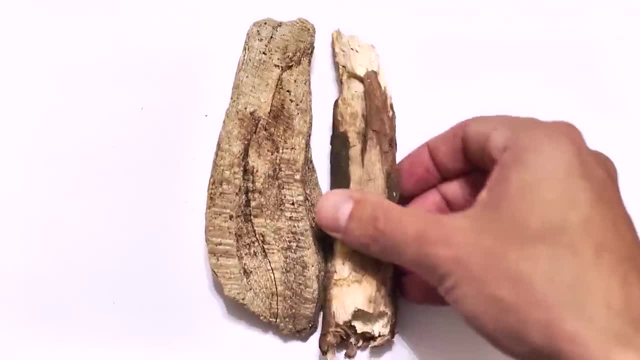 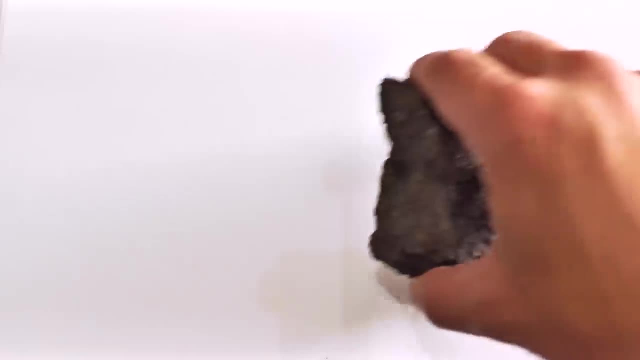 If you take a piece of wood and put it next to another piece of wood, nothing happens. And if you take a piece of granite and put it next to another rock, still nothing. But if you take this piece of iron and put it next to this other piece of iron, magic. 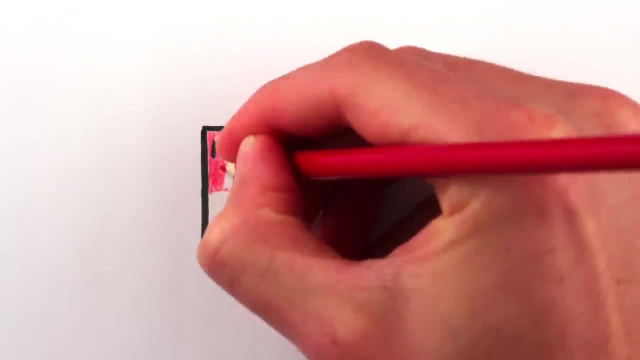 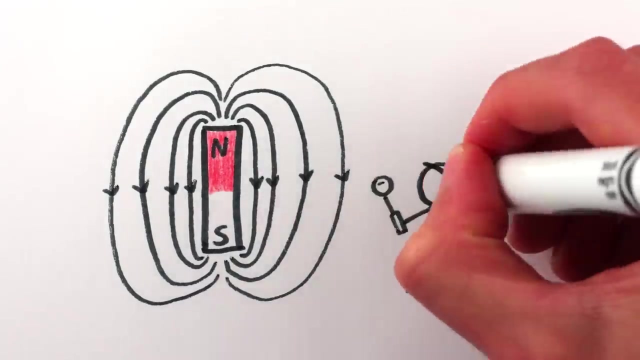 I mean magnet. Magnetic objects are able to magically attract at long distances because they generate magnetic fields that extend invisibly out beyond the object. But the mystery is this: Where do magnetic fields come from? Well, that's easy, Henry. We've known for a long time that electricity and magnetism 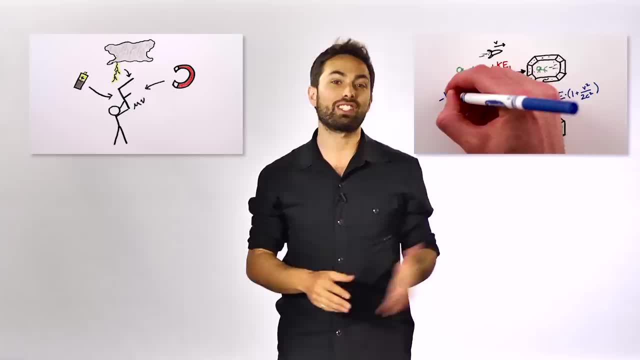 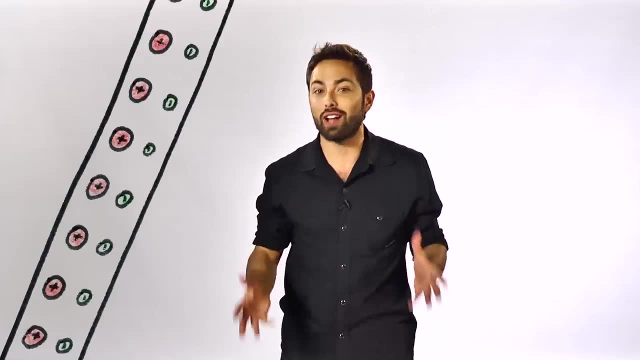 are really just two sides of the same coin, kind of like mass and energy or time and space. They can be transformed into one another And in fact a magnetic field is just what an electric field becomes when an electrically charged object starts moving. 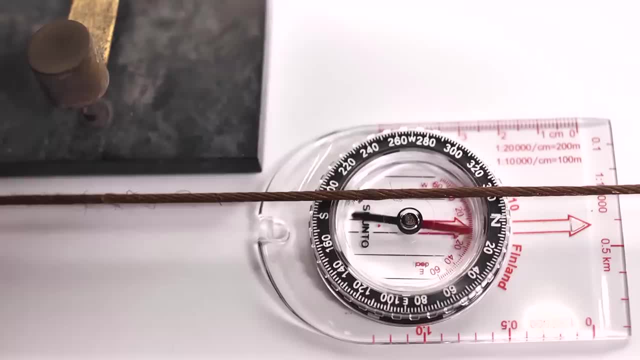 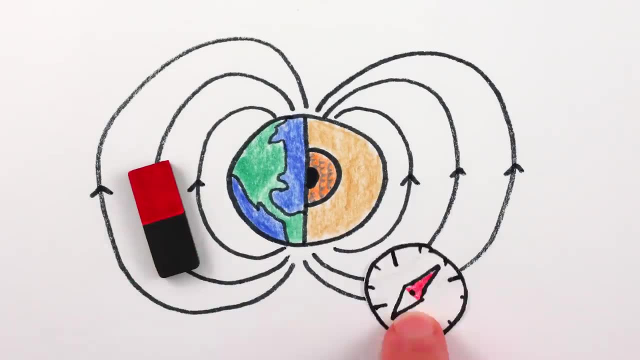 That makes sense for explaining why a current of electrons flowing through a wire causes this compass needle to move, or how currents in the Earth's outer core generate the geomagnetic field. But a bar magnet or the compass needle itself are just pieces of metal without any electrical current running through them.